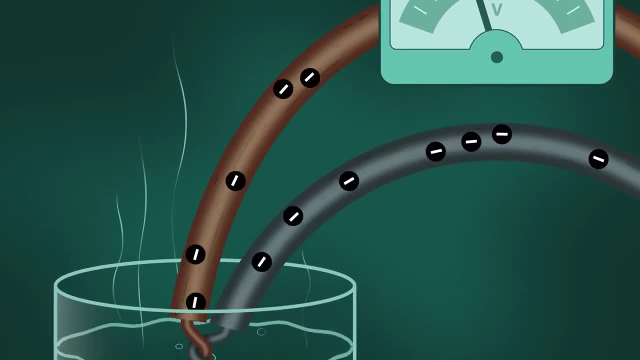 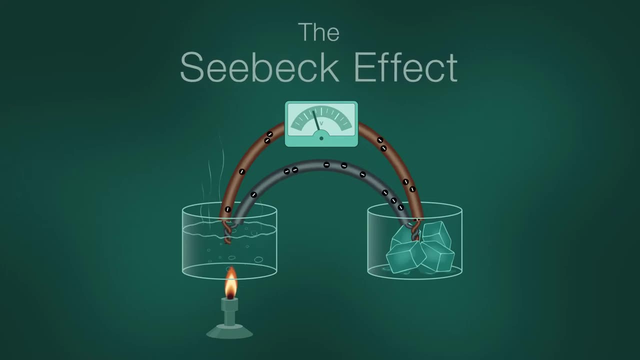 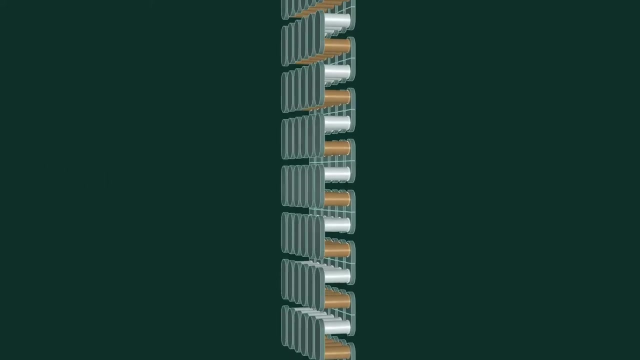 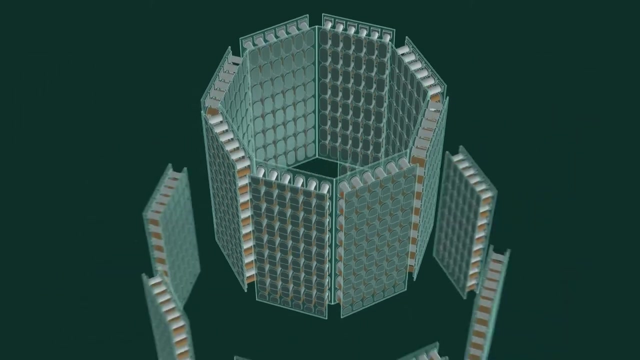 heat source, or the hot side to the colder side. We now call this process of producing electricity the Seebeck effect. Today we use the term thermocouple to describe the hundreds of small pairs of junctions made from different conducting materials that take advantage of this property. We now know that. 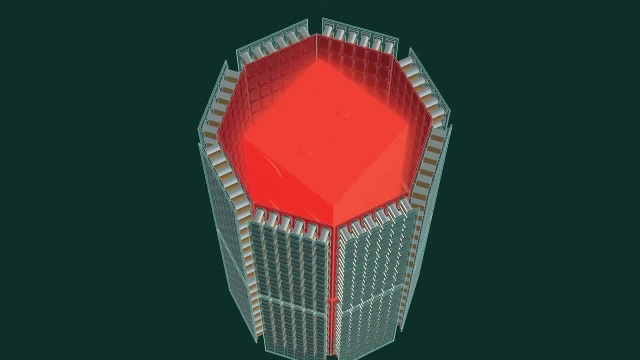 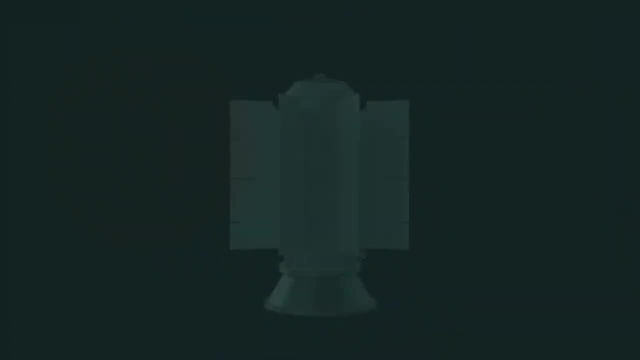 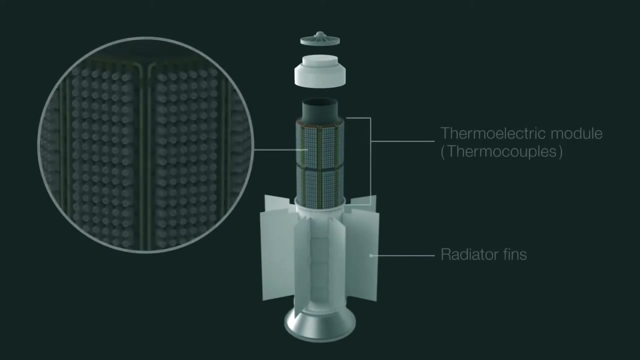 the greater the difference in temperature between the hot side and cold side, the greater amount of power that can be generated Inside a radioisotope thermoelectric generator, or RTG. these thermocouples are strung together in a long series so they can generate a steady 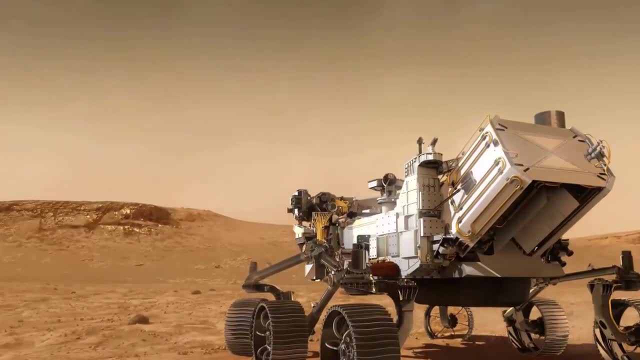 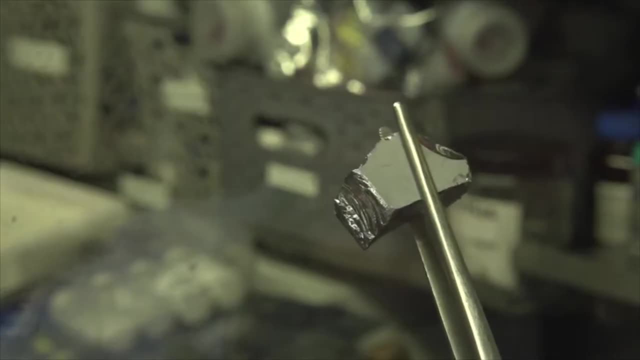 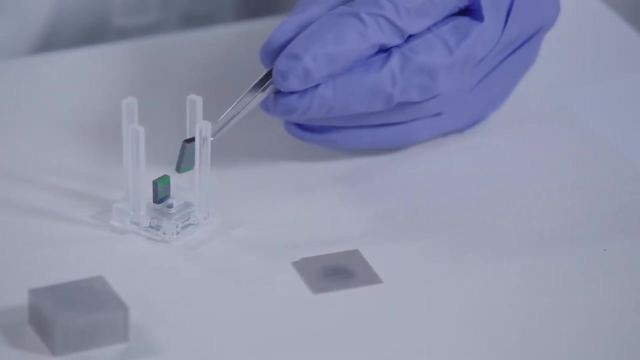 current of electricity that can provide robotic spacecraft with the power they need to operate. Some of the specific materials used in RTGs are selected because they can conduct electricity as well as maintain a hot and a cold side. Seebeck used copper and bismuth in his experiments. 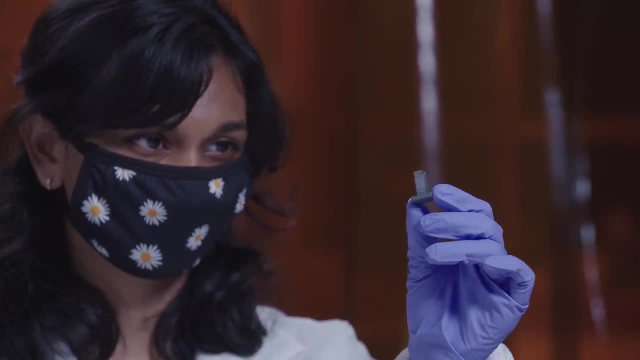 Today we use lead, telluride and copper. The thermocouple is made of copper and bismuth. The thermocouple is made of copper and bismuth. The thermocouple is made of copper and bismuth. These materials are part of a family of compounds known as semi-conductors. 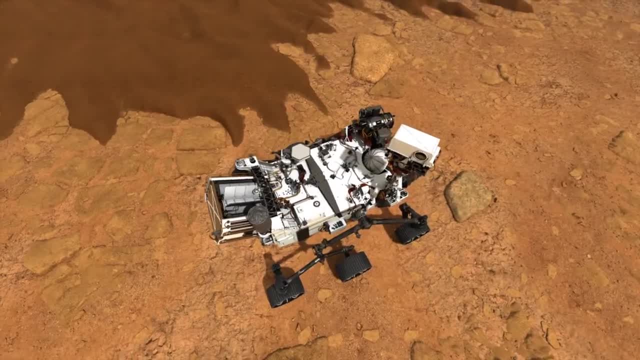 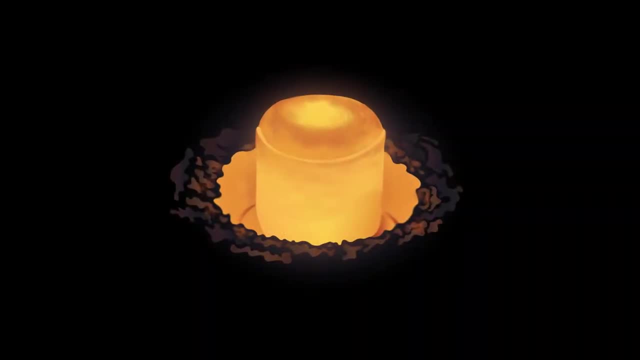 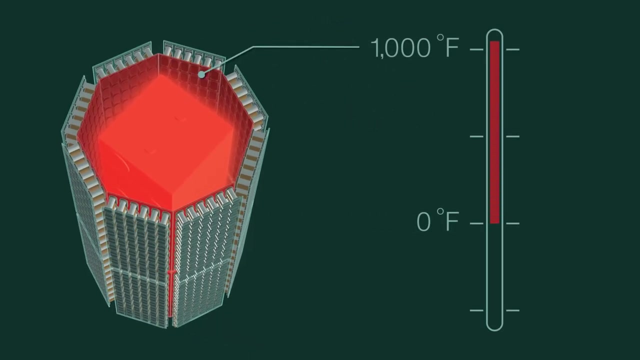 In the RTGs built by the US Department of Energy and used by NASA. the hot side is provided by the heat energy emitted from the natural radioactive decay of plutonium dioxide. The hot side of the thermocouples can be more than a thousand degrees Fahrenheit or 500. 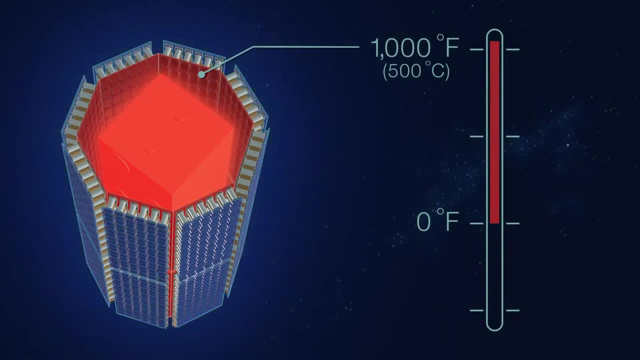 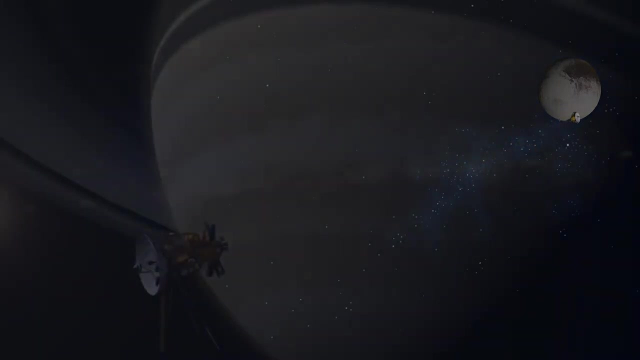 degrees Celsius. The cold side faces out into space or into the atmosphere of a planet or moon where the temperature can be well below zero. In addition, since no moving parts are involved, the thermoelectric effect is extremely reliable. Over the years, the thousands of thermocouples in NASA's nuclear batteries 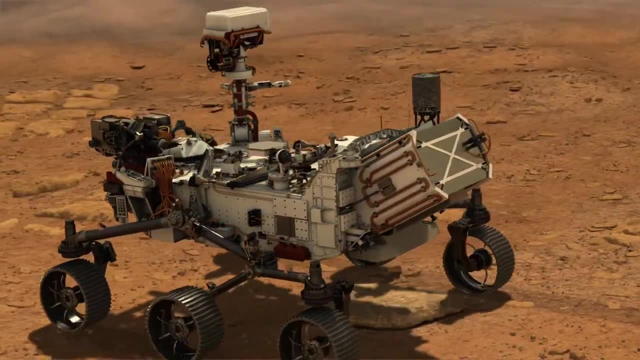 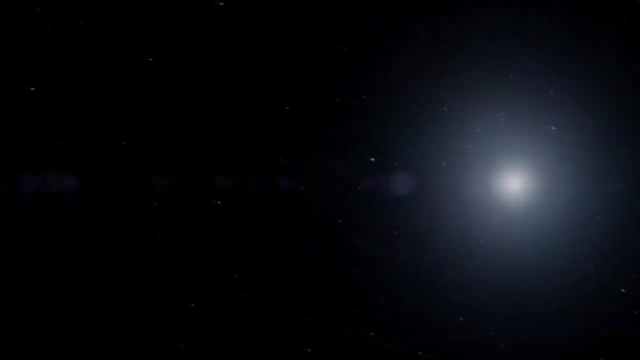 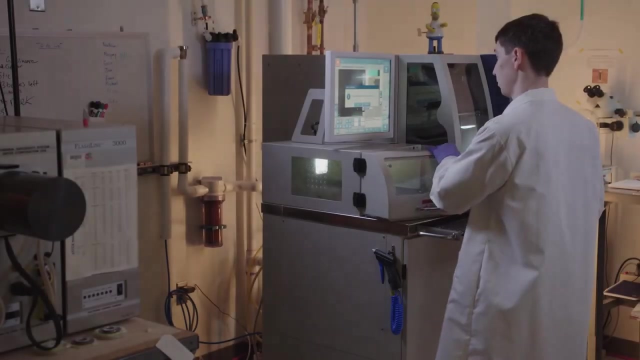 have performed without any noticeable failures in all of the two dozen missions in which they've been used. For example, NASA's two Voyager space probes powered by RTGs have been carrying on steadily since their launch back in 1977.. By using new, more CBAC-friendly materials.